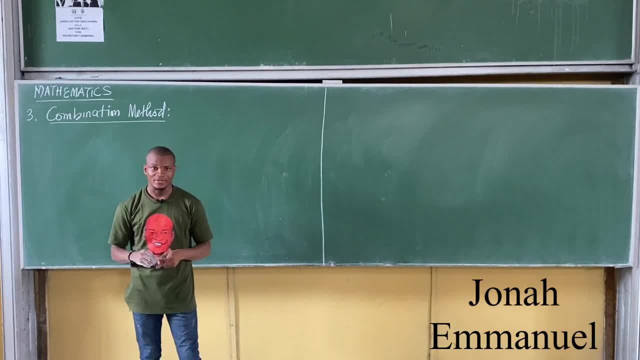 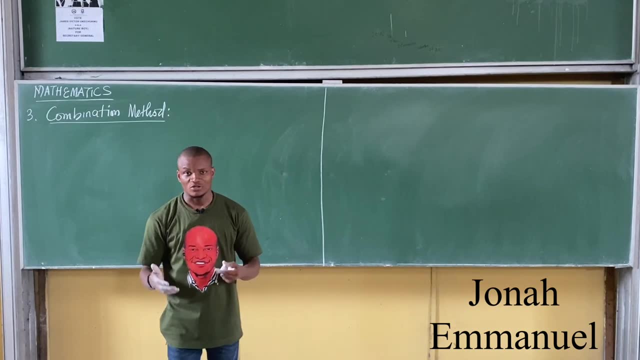 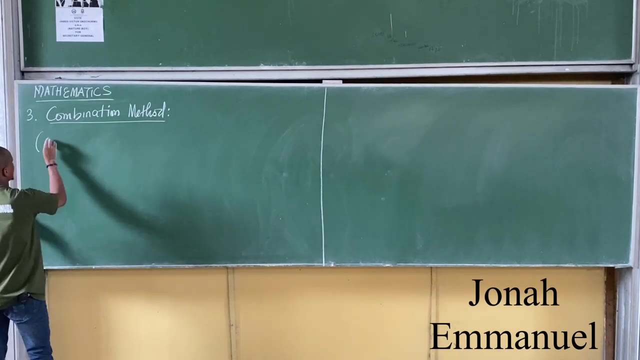 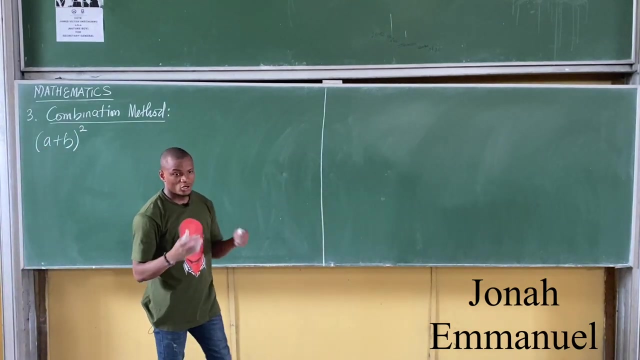 So it gives the coefficient of terms in a binomial expansion. So how do you expand terms using combination method? So here's how it goes. Let's say I'm giving the terms, Let's use our a plus b. Let's say I'm giving a plus b over 2 and I'm asked to expand this via combination method. What do I do? 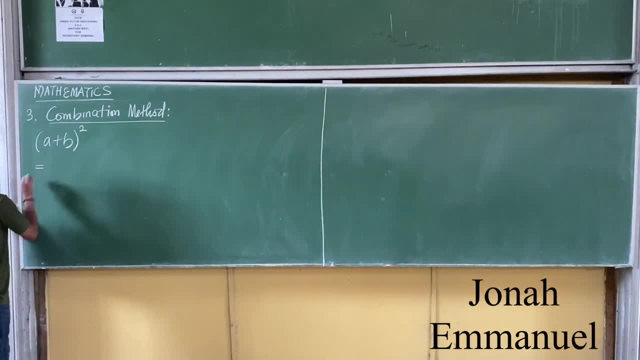 So this will be equal to The idea. is this? My part here is 2.. So the terms 2 combination start with 0. So 2 combination always start with 0.. Now bringing back the idea of Pascal's triangle. 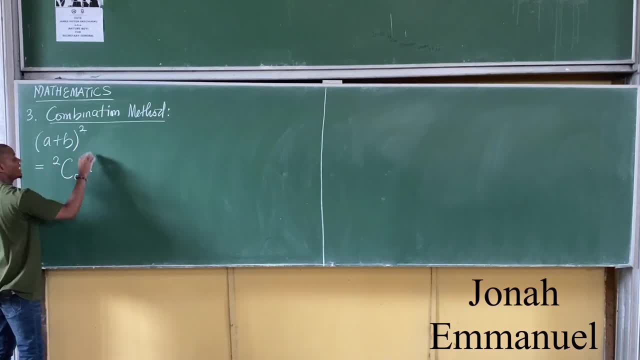 When we say, the first term takes all the part and the second term is left with nothing. So I have this Plus The second term becomes the same thing here. 2 combination Here was 0. Increase it to 1. So I have 1.. 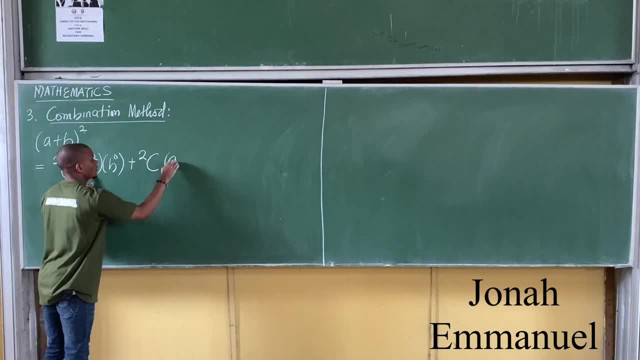 For here I have a. Reduce this part by 1.. As we did in Pascal's triangle. It becomes a to the power of 1.. I'm having b This to the power of 0. Increase it by 1.. 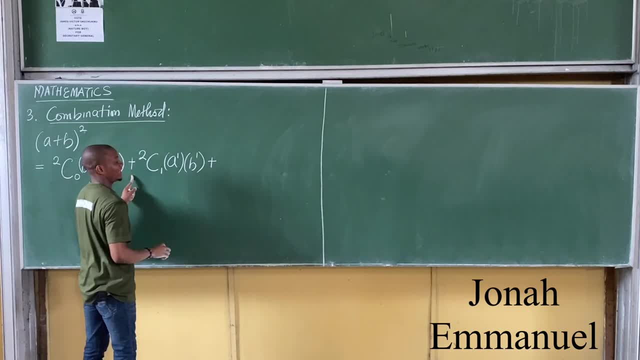 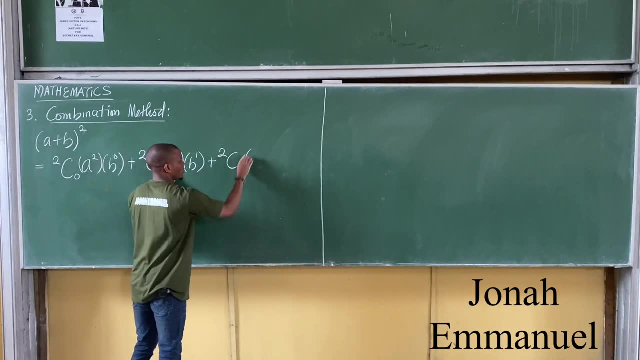 It becomes 1.. Plus my next step, The same thing here: 2 combination, 2.. Of course, reduce this by 1.. It becomes a to the power of 0. And finally, I have b. Increase this by 1.. 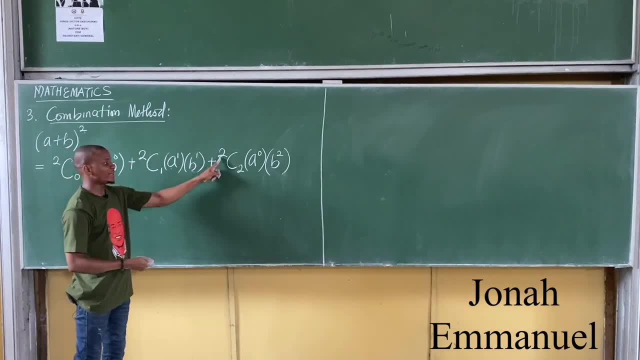 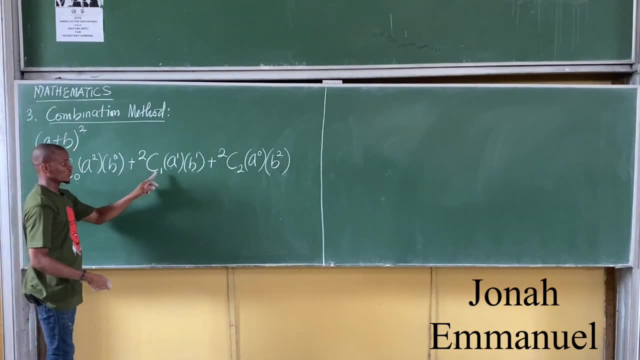 It becomes a to the power of 2.. For combination method, you stop when these two terms are exactly the same thing. Alright, So start with 2 combination 0.. 2 combination 1.. 2 combination- 2.. Observe that this 2 will always be constant. 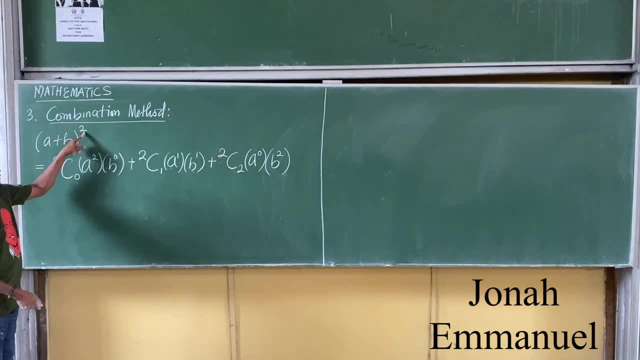 Alright, This 2 is from the power here. So, assuming my power was 3. It would have been 3, combination 0. And it is here. Alright, Let's work this out. then Let's look at the cost of combination. 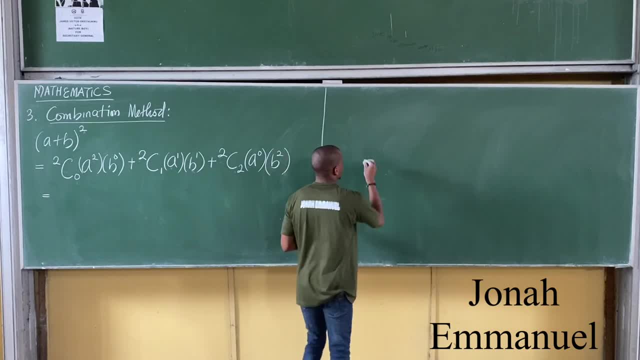 What does combination mean? Alright, Usually, if I say n combination r, from mathematical approach This is equal to n factorial all over n minus r factorial and then r factorial. This is the value of a combination. So hence, if I have 2 combination, 0.. 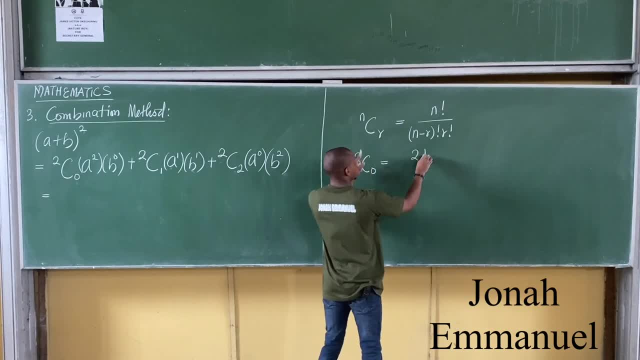 This would be equal to 2 factorial, that's n factorial all over n minus r. That becomes 2 minus 0 factorial. Then finally r factorial, That gives you 0 factorial. When we say a factorial, A factorial is simply the multiplication of 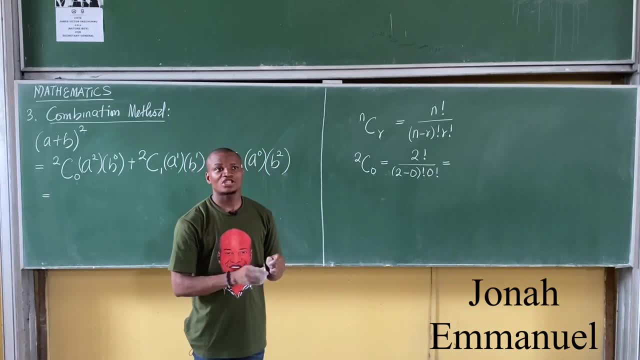 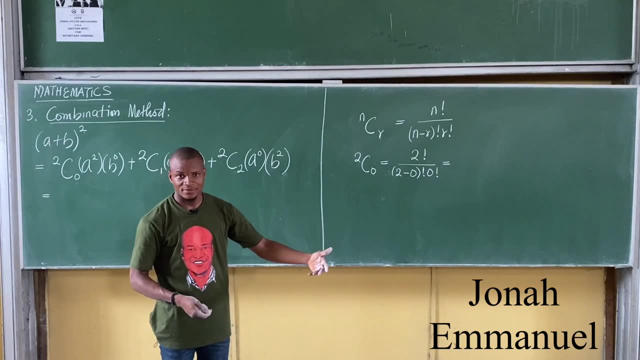 consecutive terms in descending order, such that each term differs from the previous by 1.. The multiplication of consecutive terms in descending order, such that each term differs from the previous by 1. Hence, 2 factorial is equal to 2 times 1.. That's all. 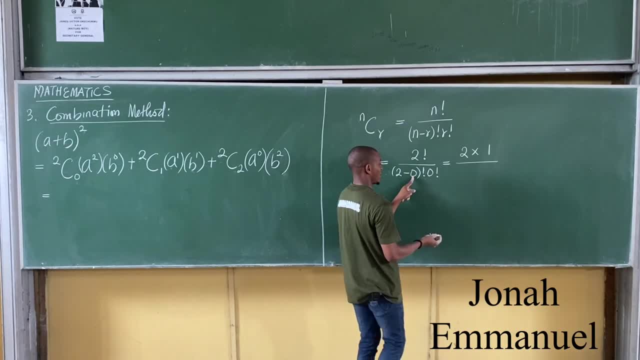 All over 2 minus 0. This is 2.. Bring this one down here. First of all. let me simplify this. first, I'm having 2 factorial all over. 2 minus 0 gives you 2 factorial and then 0 factorial. This would be equal to: 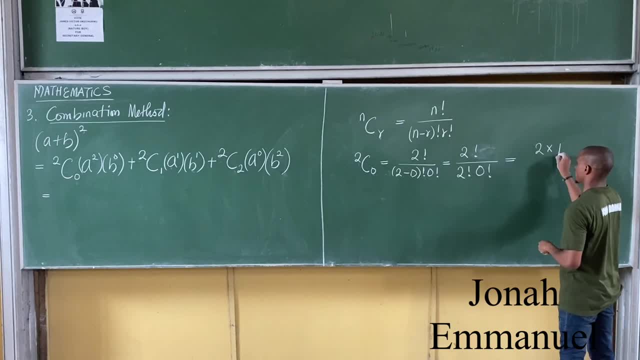 2 factorial is 2 times 1. all over. 2 factorial is 2 times 1.. 0 factorial is 1.. From here, this cancels this. It's 1: 1. That's equal to 1 times 1 is 1. All over. 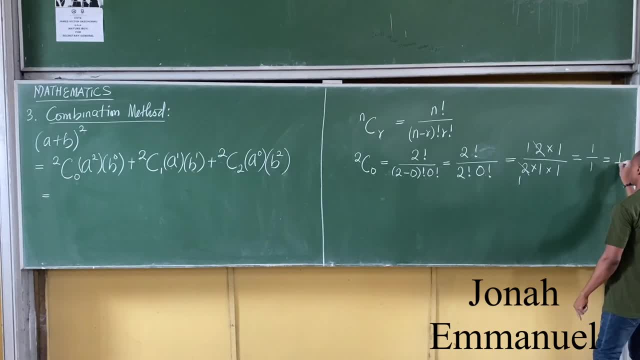 1 times 1 times 1 is 1.. 1 over 1 gives you 1.. So 2 factorial 0 is equal to 1.. Now if you want to take through this process, you can see that it becomes very lengthy to solve. So instead, 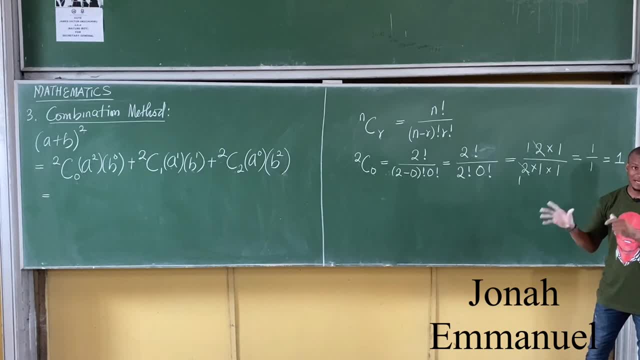 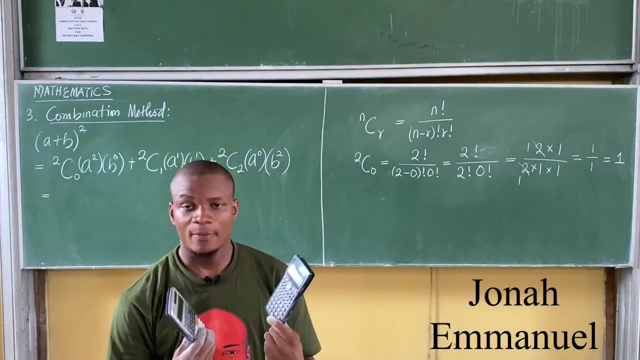 we employ the use of a calculator for that, Alright. We treat permutation and combination as a topic separately, much more later. So let's use calculator for now. Now, how do we use calculator? Let's have a look at this, Alright, So 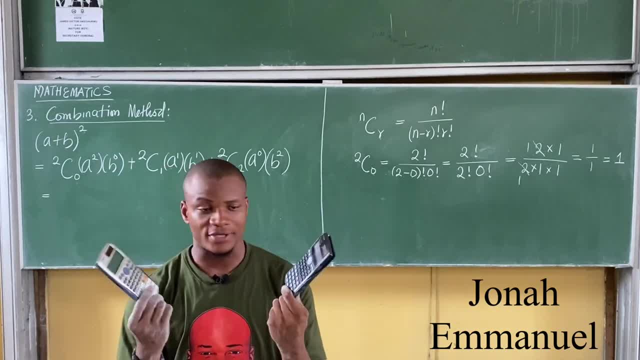 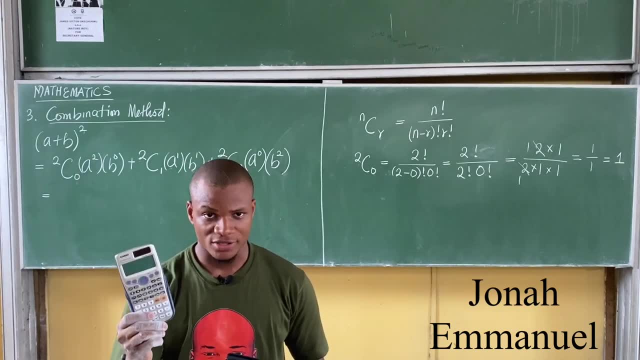 how do we use calculator in doing prevalence and combination? So I have 2 calculators here. This is Casio FX 991 MS, This is Casio FX 991 MS Plus, So we can use each of any of these to do the 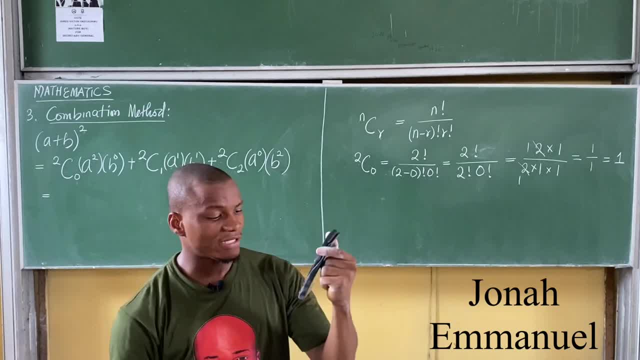 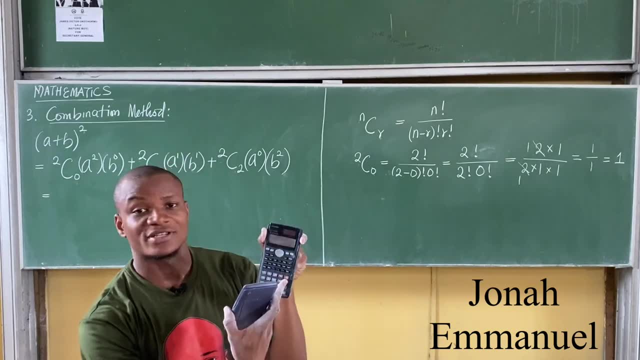 combination. Now, how do we solve combination using this? If I look at both FX 991 MS and FX 991 MS Plus. If I look at the divide button here- Also here too. If I look at the division button here and here. 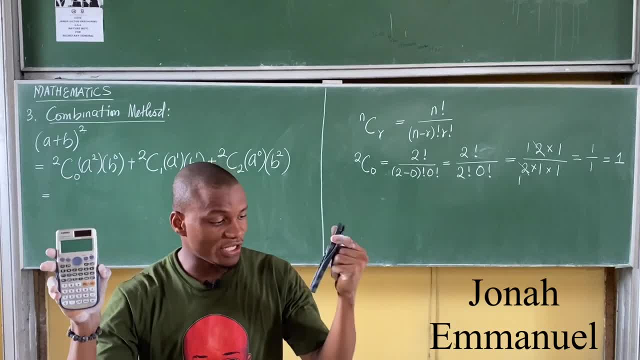 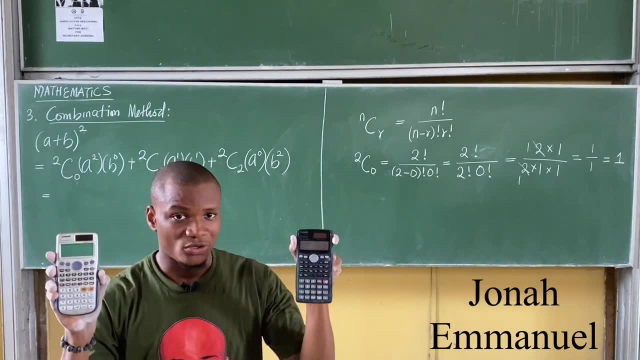 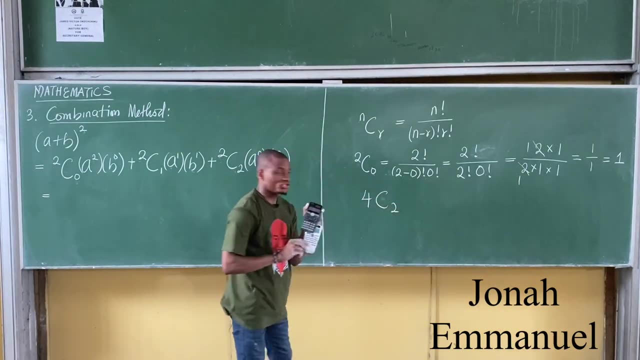 Up of it, that's on top of it you see n, combination R written in yellow. So this is how I can punch combination using the calculator. So let's say I want to punch, for instance, 4 combination 2 using either this or this. What do I do? 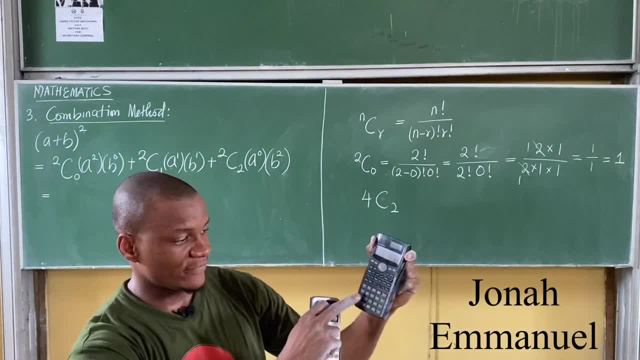 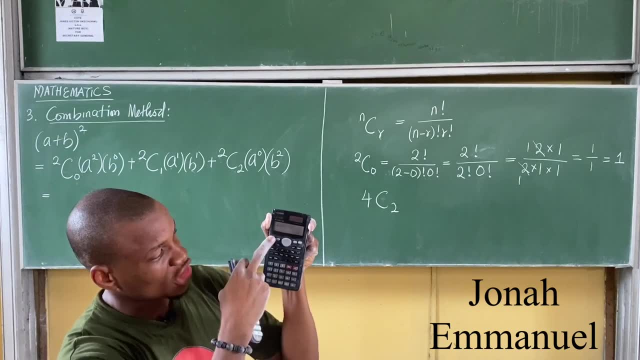 It's as easy as this, So I'll punch 4.. That gives you 4 here. Next up combination is up of divide sign. So you press shift and divide. When you press shift and divide, you see 4C there. This C means: 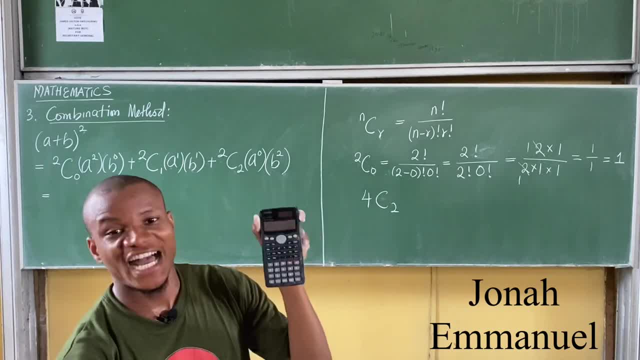 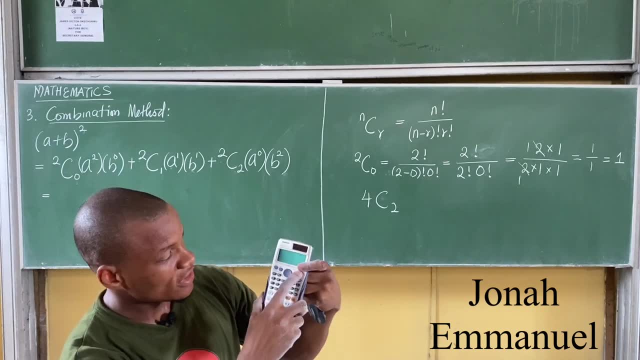 combination, Then press 2.. So it's equal to. I have my answer as 6.. Alright, Do the same thing here. Same thing with FX 991 MS Plus. So this gives you 4. Shift, press divide, You see. 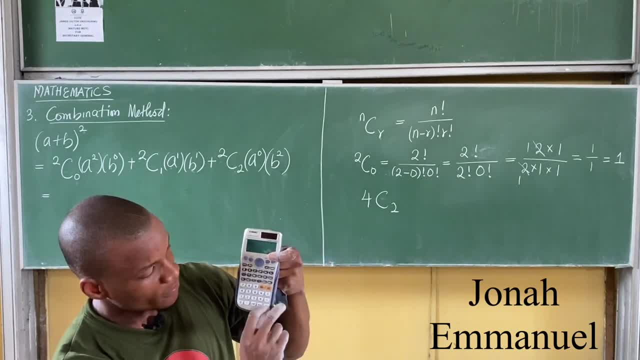 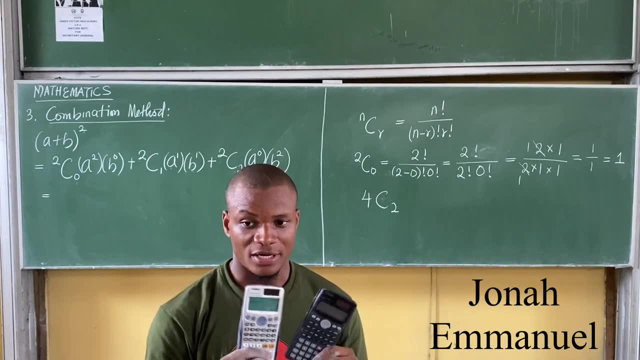 4C, Press 2. That's 4 combination, 2. Press equal to you have 6.. So this is how you do combination using any of these calculators. We'll go back to this and they'll give me the answer. 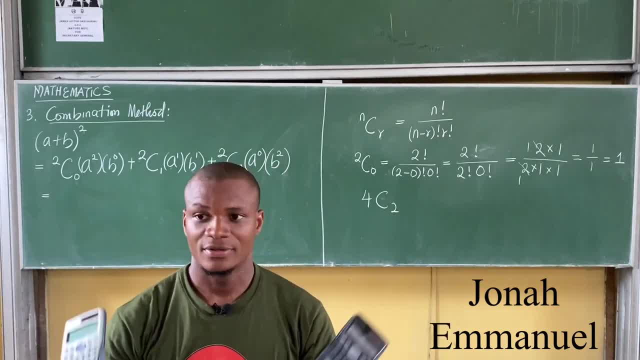 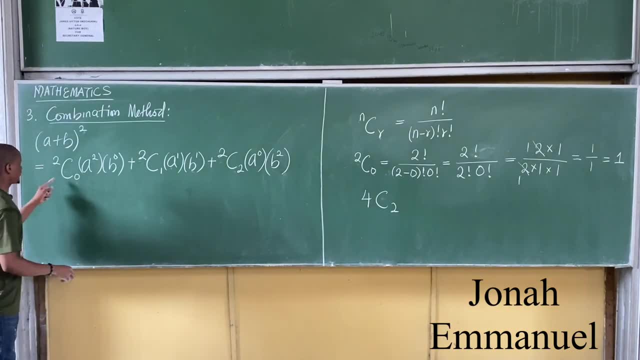 of each of them using calculators. Alright, So just punch and tell me your answer, please. Alright, So please. What about 2 combination 0?? We have this. what Check? 2 combination 0.. What do you have here? 1. 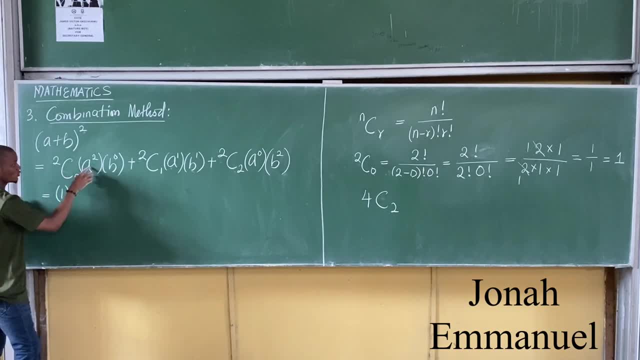 So it becomes 1 here. That's from here, And so this gives you A squared B to the power. 0 is 1.. Plus 2 combination 1, here You have your answer as 2.. Alright, A to the power. 1 is A. 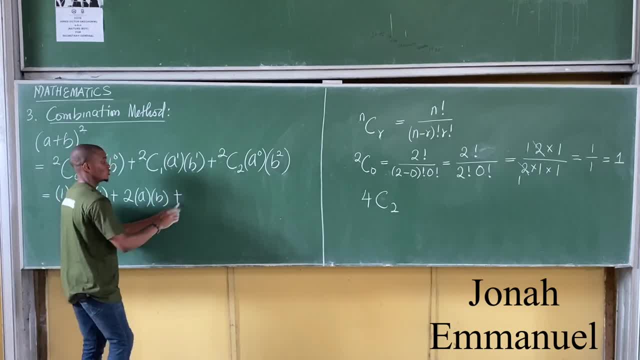 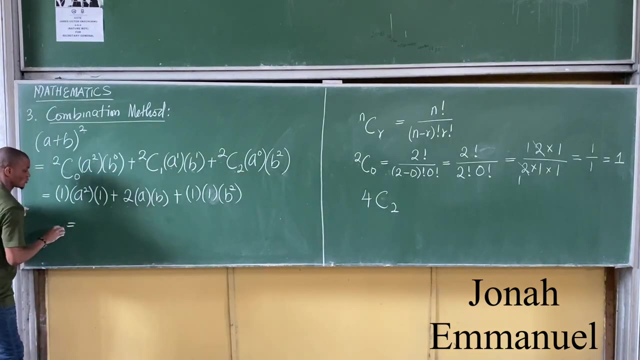 B to the power. 1 is B Plus 2 combination: 2. Report you that you have 1.. So I have 1 into A to the power. 0 is 1.. Then next up, I have A squared. So this is now equal to. 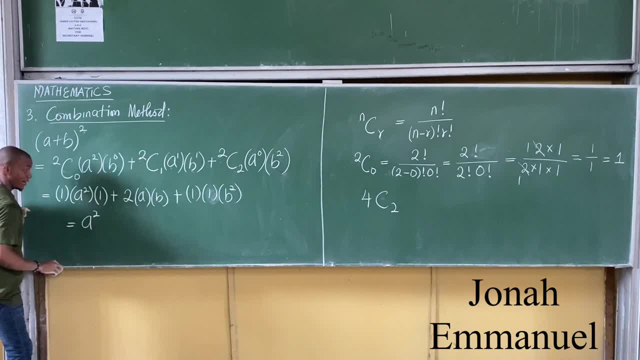 1 times A squared times 1 gives A squared Plus next up 2AB. 2 times A times B: 2AB plus 1 times 1 times B squared, That's B squared. So this becomes my answer after using. 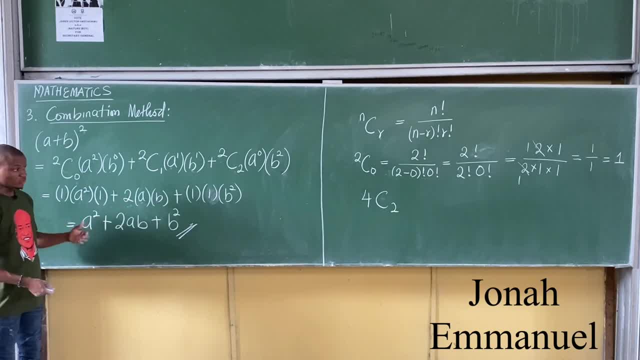 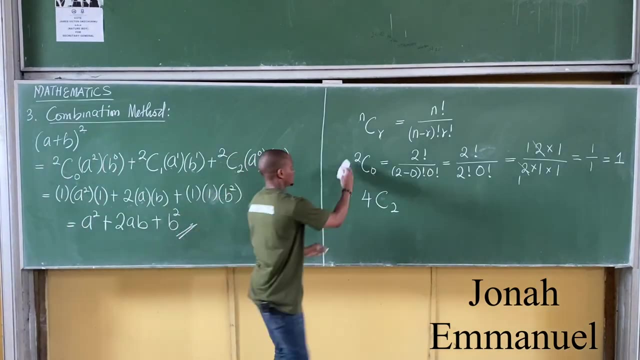 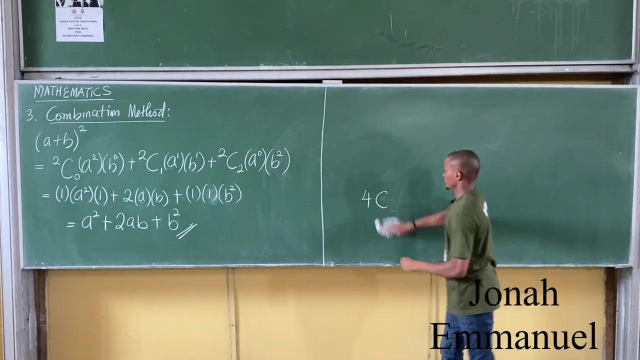 combination method. So here I have the same answer when I use my general expression method, When I use Pascal's triangle and when I use combination method. We'll take just one more example of combination method and we're done. Alright, Let's see. 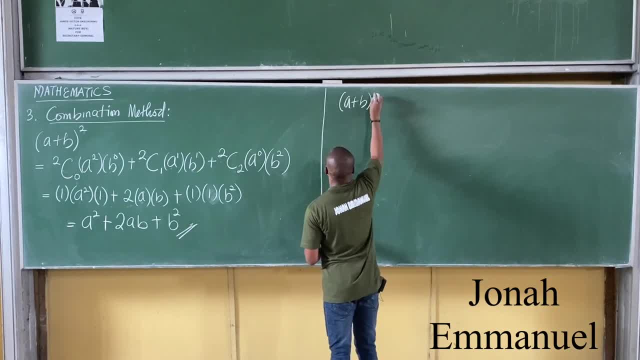 for a second example, Let's say A plus B to the power 5, using combination method. So this will be equal to. we said this: the power here, That's 5. combination. start with 0. combination 0 into this term. A takes all the power. 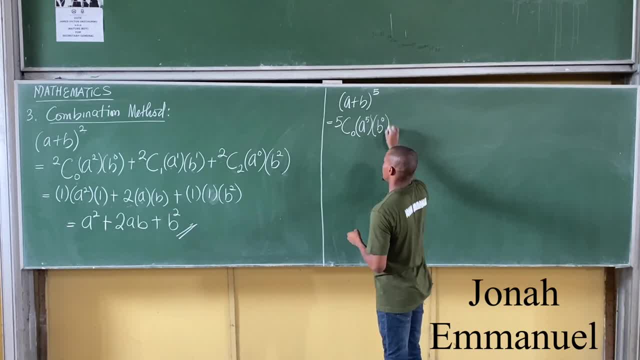 5. B is left with 0 or nothing. Plus this becomes 5 combination. from 0 increase to 1, as we did here, Becomes 5 combination. 1 into this gives you A to the power. reduced by 1, that becomes 4. Increase. 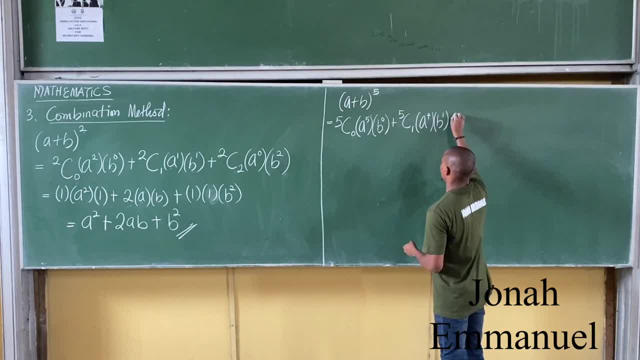 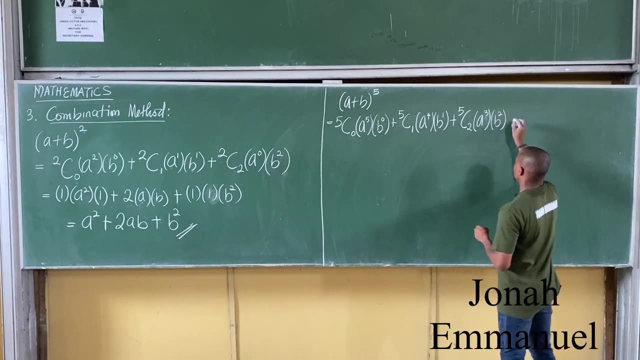 by 1 becomes B to the power 1.. Okay, Plus 5 combination: 2 into reduced by 1. A to the power. 4 to the power 3: increase the power by 1 becomes B squared Plus 5 combination from 2 to 3. 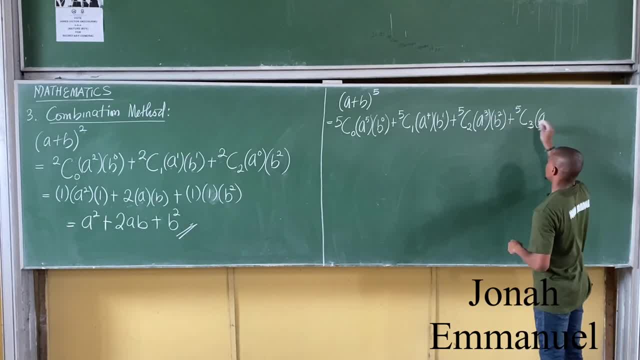 that becomes A to the power. 3 minus 1 is 2.. B into 2 plus 1 is 3 plus my next. that becomes 5 combination, 4.. So I have A to the power 3, 1.. I'm using this. it becomes: 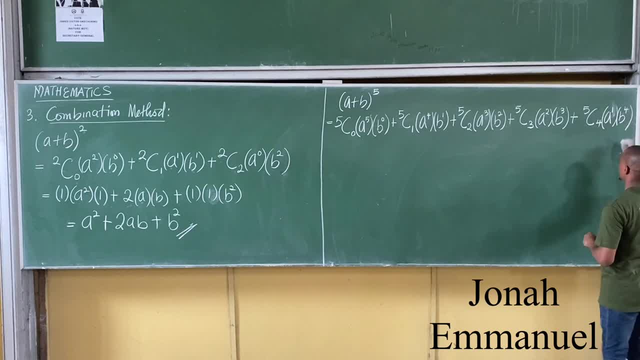 1.. Then B to the power 4. 1 final term comes to plus 5 combination 5.. That gives A to the power 0, then B to the power 5.. Alright, This is now equal to 5 combination. 0 gives you 1. 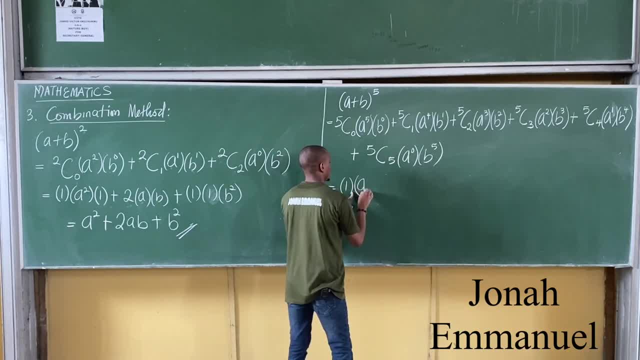 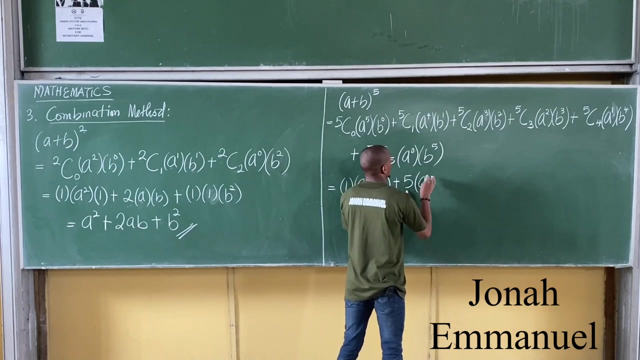 into A to the power, 5 into B to the power. 0 gives you 1 plus 5. combination 1 put together that's 5, 5. A to the power, 4, B to the power. 1 is B plus. this gives me 10. 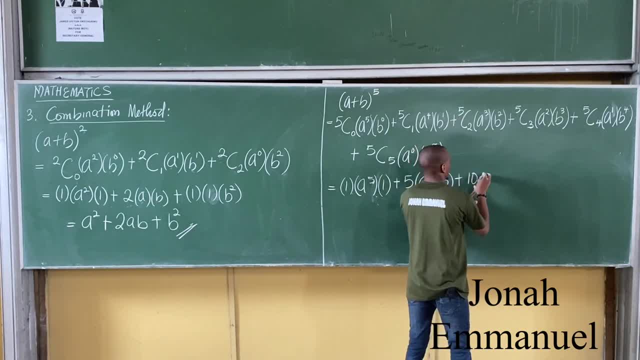 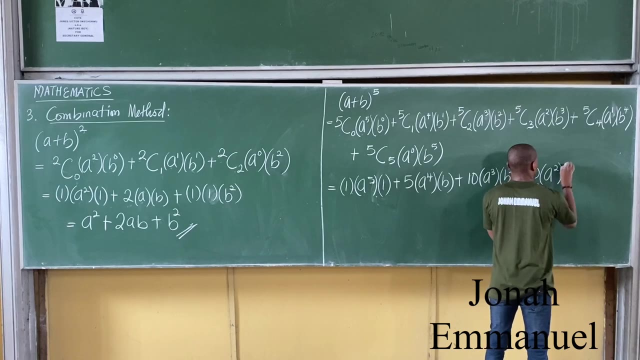 5. combination 2 gives you 10 into A cubed B squared Plus 5. combination 3 gives you 10: 10 A squared B cubed plus 5. combination 4 gives 5 into A to the power 1 is A. 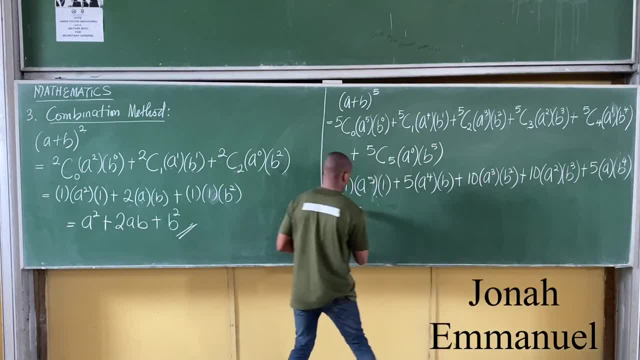 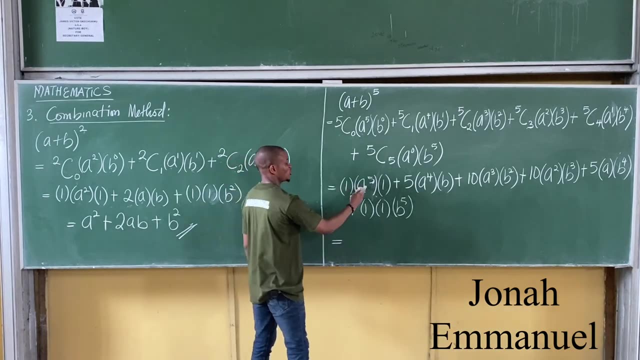 then B to the power 4 plus 5. combination 5 gives 1 into A to the power. 0 is 1. and then B to the power 5.. Alright, So if I want to reduce this issue, 1 times A to the power 5. 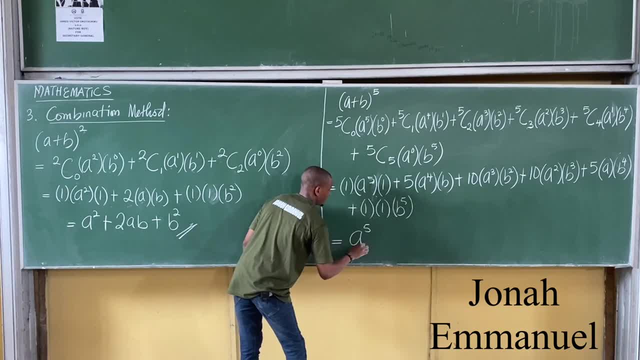 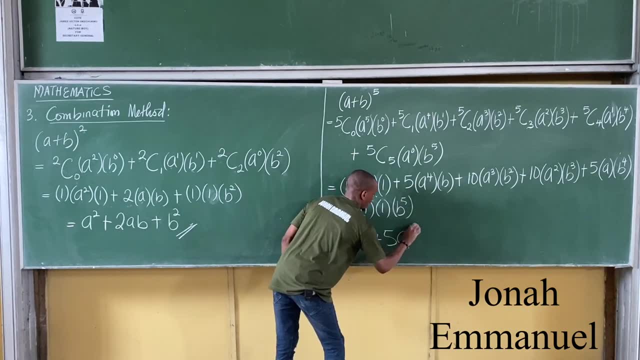 times A. that gives you A to the power 5 plus 5 A to the power 4 B. I have 5 A to the power 4 B plus I have 10 A to the power 3 B squared, 10 A cubed B squared plus. 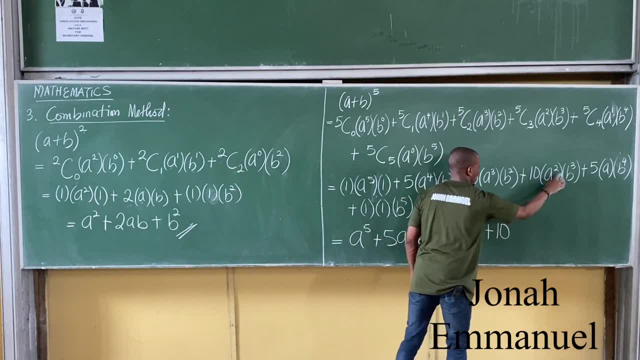 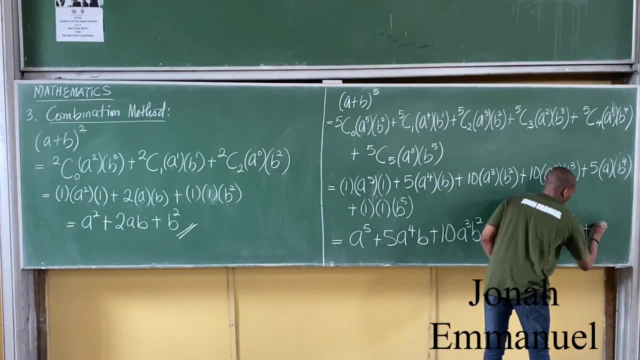 I have 10 A squared B cubed A squared B cubed plus. I have 5 A to the power 4, 5 A B to the power 4 plus 1 times 1 is 1 plus B to the power 5. So this is how we solve problems. 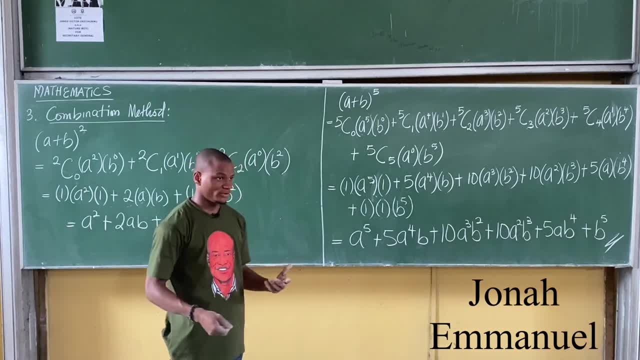 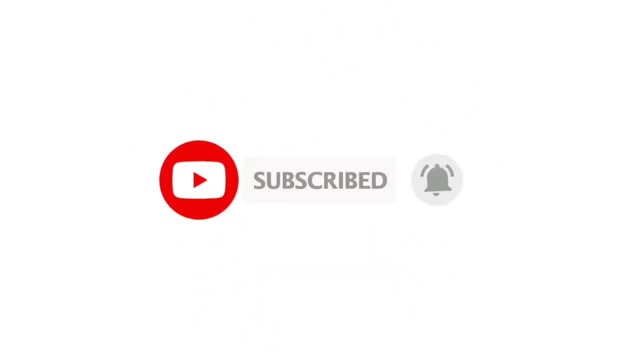 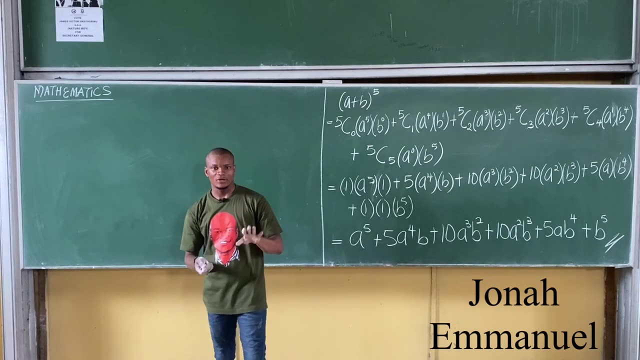 using combination method. So this is how this is done. Alright, So if we will proceed to something else, why do we have? we said we have 3 methods in solving binomial expansion: the general expansion method, the Pascal's triangle and then the combination method. 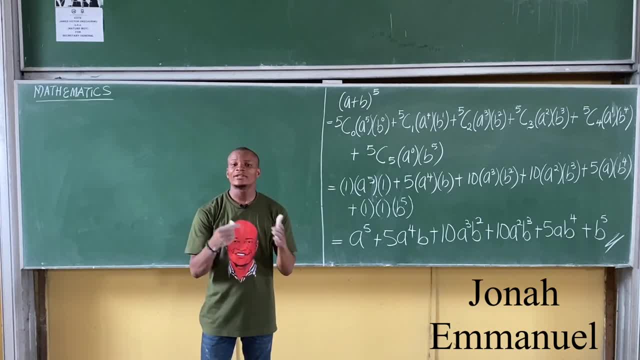 Now, if I have general expansion method, why the need for Pascal's triangle? If Pascal's triangle can give me a fast approach to solving problems, why the need for combination method? So I will explain the need for all of these other methods aside from the previous one. 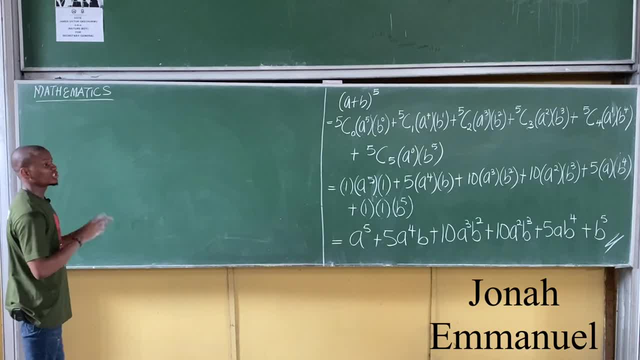 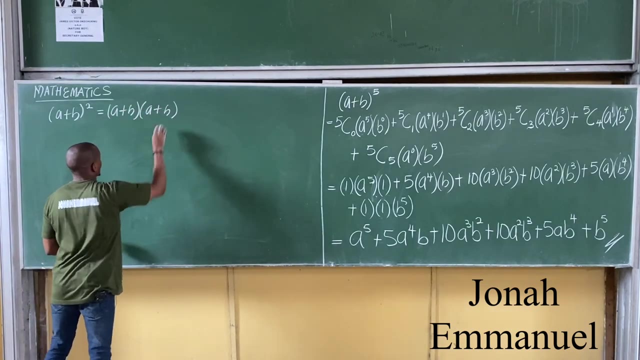 Now let's talk about the first method. For the first method we said is the general expansion method. I said for general expansion method, if I am given A plus B to the power 2, this is equal to A plus B multiplied A plus B. Now try to imagine. 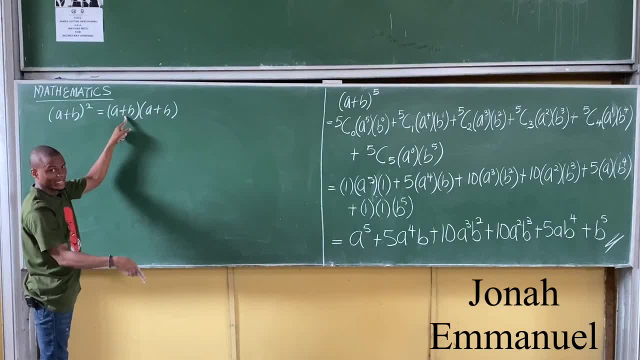 and I said for this case here all of the terms in the first bracket to multiplying all the terms in the second bracket, as we did in the previous class. But let's try to imagine this was A plus B to the power, let's say 22, for instance. 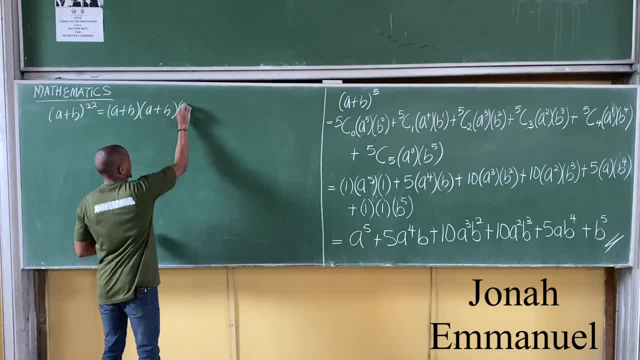 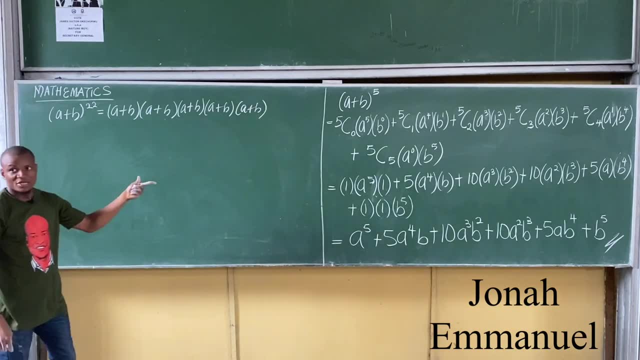 So this would be A plus B, multiplying A plus B, multiplying A plus B, multiplying A plus B to the power 22 becomes 2 comparison to handle Now using general method for this. while it's quite possible, it's very difficult. So this becomes the limitation. 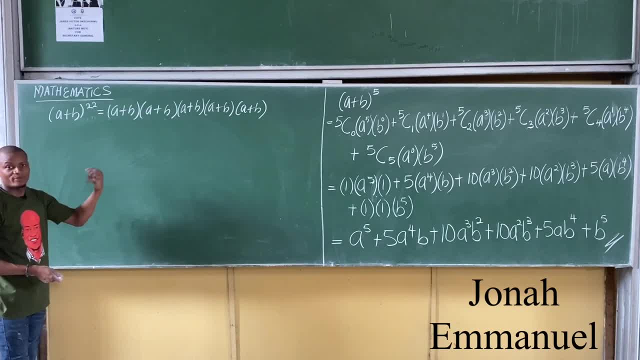 to the general expansion method. So general expansion method can be used for just small positive index. small positive index like 2, 3,, 4, 5, or you can even do 6, but that would still be very lengthy. So this becomes the limitation. 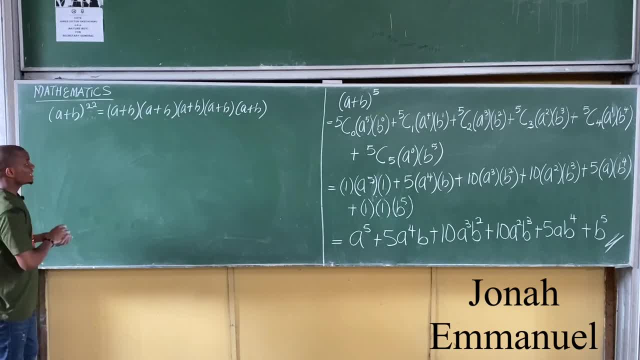 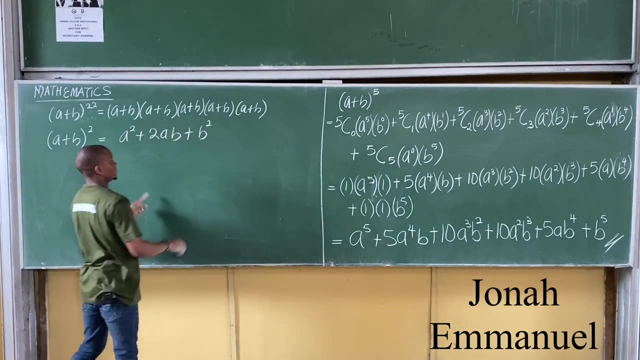 of the general expansion method. Now, next option, let's consider Pascal's Triangle. Now we said, Pascal's Triangle helps us to solve this. Pascal, something of this. We just simply need to know the coefficient for each of the terms. Now here's where Pascal's Triangle becomes. 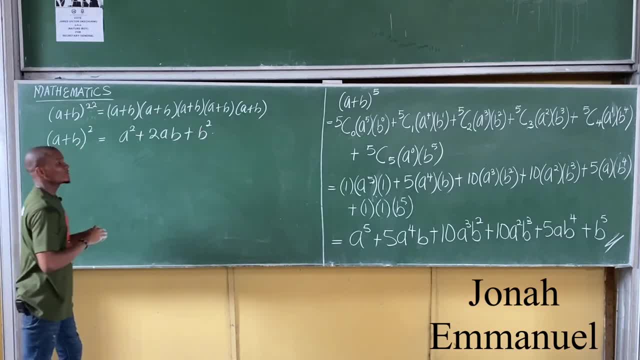 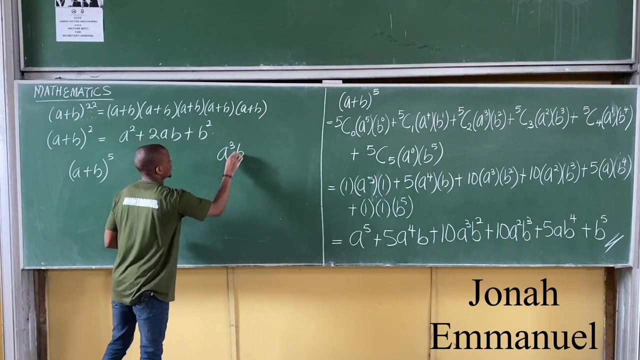 an indication. So imagine this Now, imagine I'm asked to find the coefficient of A plus B to the power, let's say 5, for instance, and I'm asked to. just the question is this now, Simply find the coefficient of, let's say, A cubed, B squared. 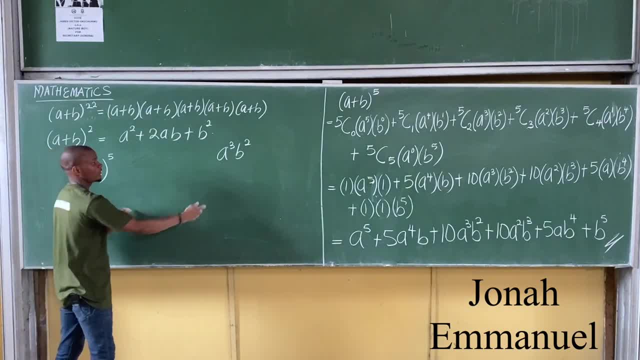 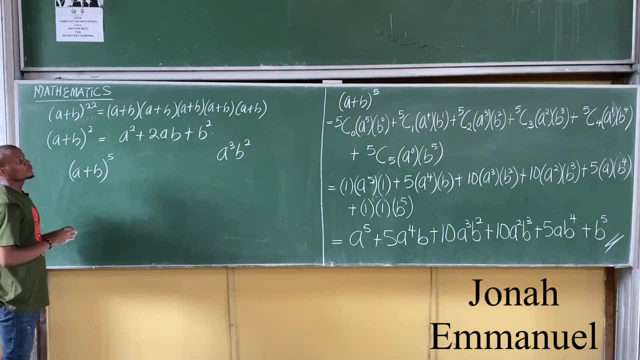 right. Find the coefficient of A cubed B squared in the expansion of A plus B to the power 5.. Now using Pascal's Triangle. here you have to expand everything first before you find the coefficient, which is very tasky. With combination method I can easily. 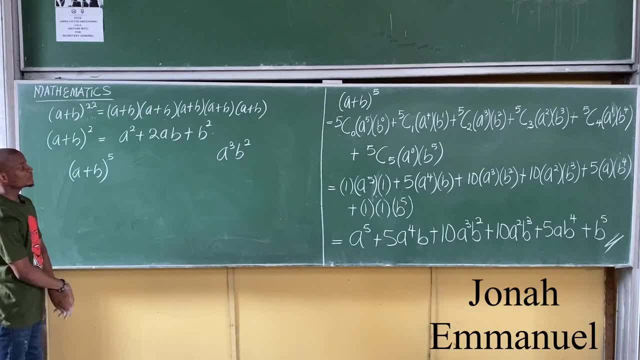 get this done right. My first ask would be: if I'm asked to find the coefficient of A cubed B squared in this, I would ask myself: is it possible, or do we have a term such as this? The answer would be yes. How do I know? 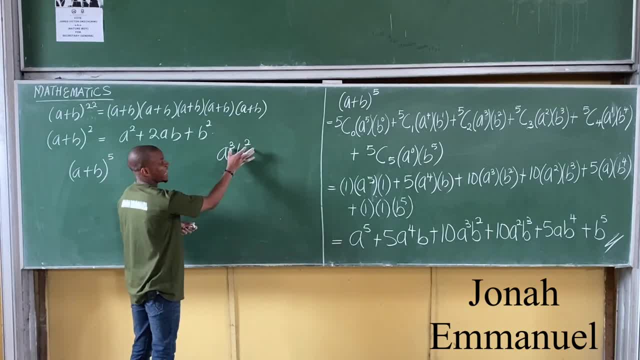 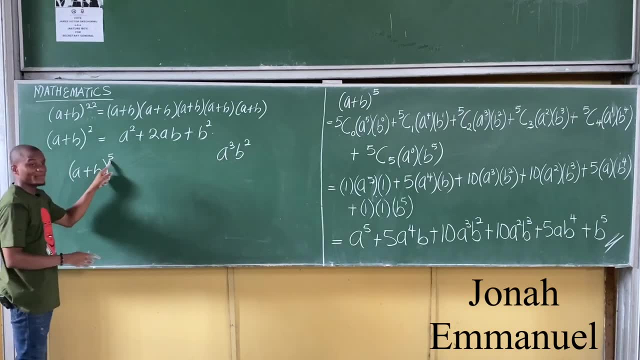 We said, when it comes to volume expansion, each of the terms, if I add the power, it should be equal to the given power. So if I add 3 plus 2 here, it gives you 5. that means a term such as this exists. Now, if I was asked to find the 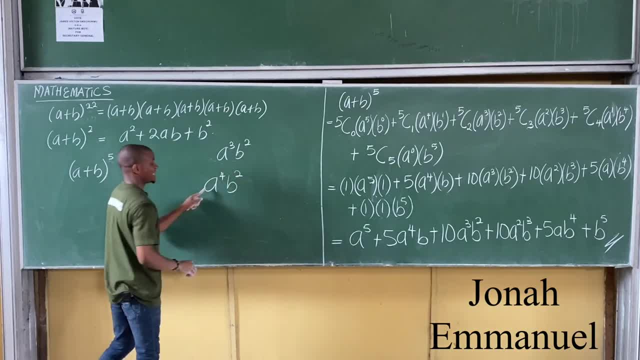 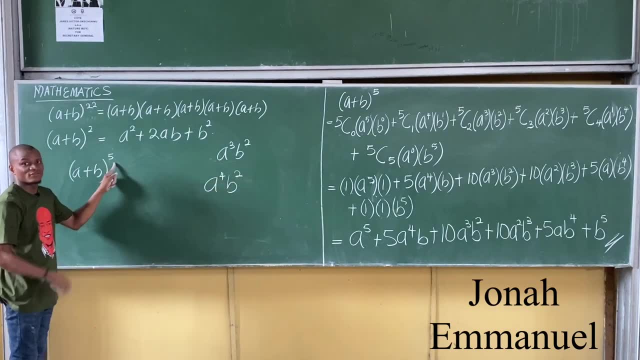 coefficient of, let's say, A cubed by 4, B squared. in the expansion of this, I would know it does not exist because 4 plus 2 gives you 6. my part here is 5. so it does not exist. it's not possible. 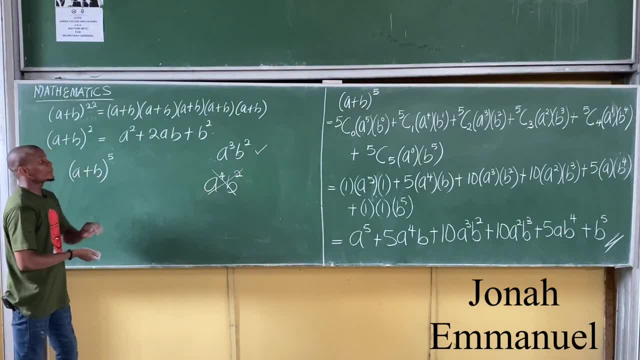 So this would not exist. why this would not exist? Now, if I'm to approach this question using Pascal's triangle, I would have to first of all get all my terms before I pick out the value. that becomes a bit lengthy if I'm to approach this. 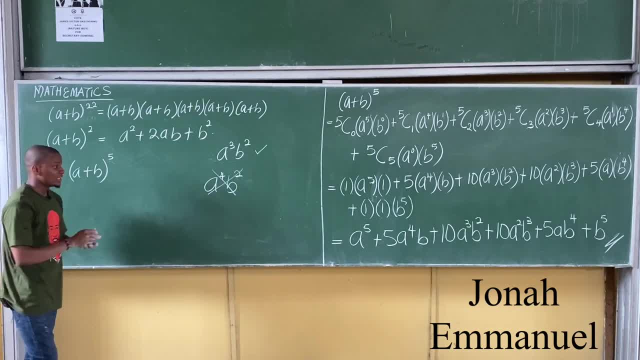 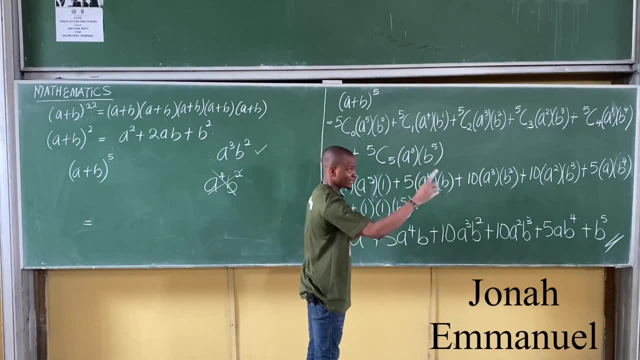 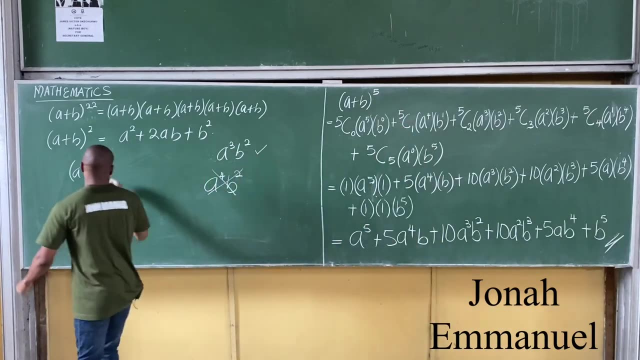 using the convolution method. it becomes very easy now using the convolution method. what do I get? If you observe my convolution method, what do you observe? is this? this one here is constant. it's always different, so it becomes. I will start this combination now. observe this, please. 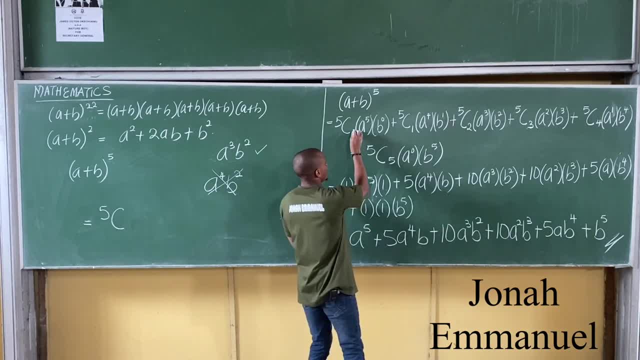 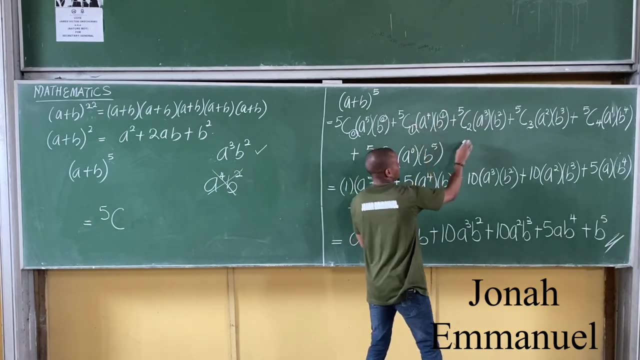 also observe that, when it comes to using the convolution method, the value here is always equal to the part of the second term. my second term here is this: the part is 0. my second term here is B, the part is 1. 1 and 1. 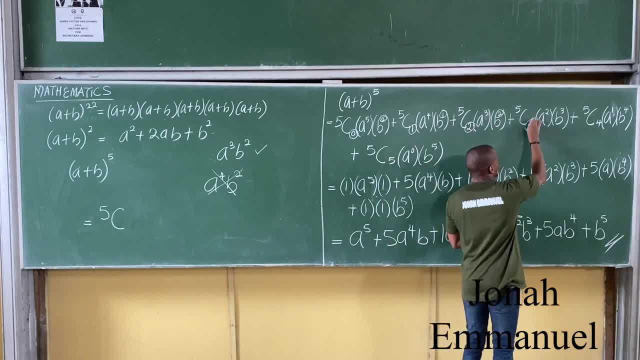 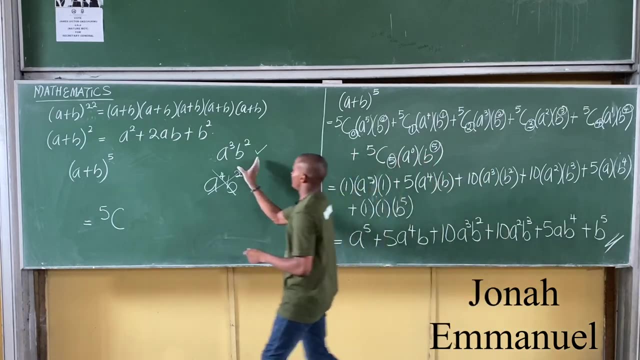 here 2 and 2, same thing here 3 and 3. also here 4 and 4, same thing here 5 and 5. that means the term that will be here is equal to the part of the second term, so if I'm taking this term here, 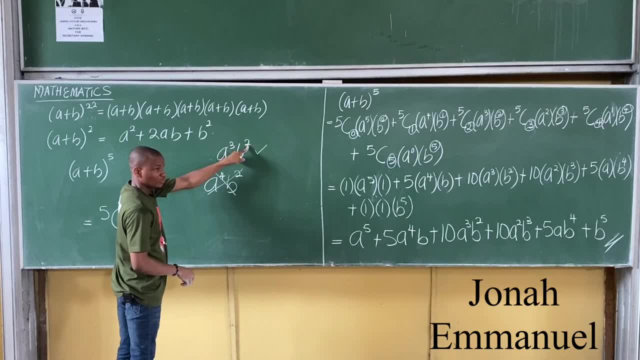 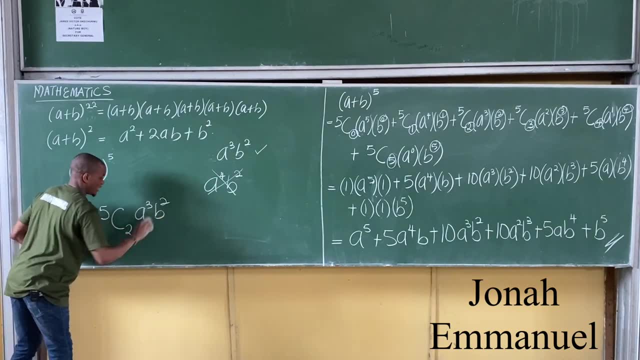 my second term is B. the part here is 2, so hence 2 again becomes 2. bring down this term: a cubed b squared. if I crunch 5 convolution 2, it gives you 10 a cubed b squared. so hence, without multiplication, you can see that. 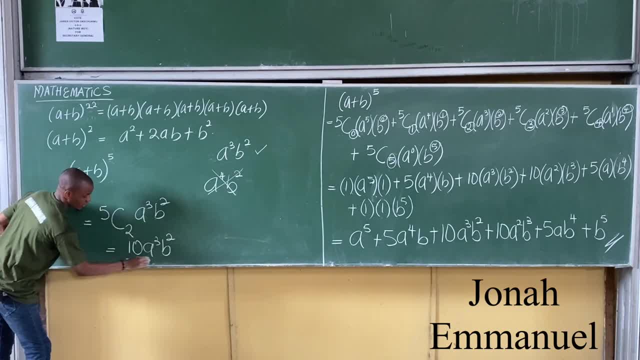 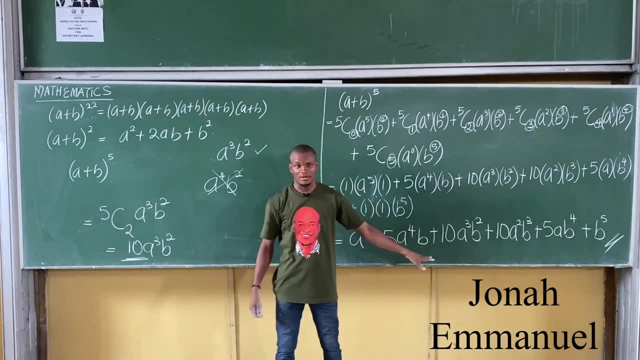 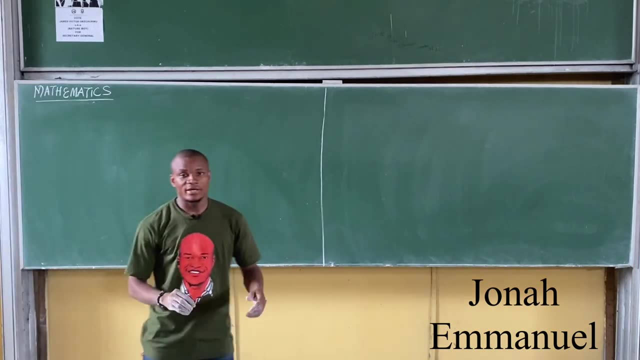 a cubed b squared in this expansion is 10 and that's what we have here. so it becomes a short cost average in getting that answer. so that's like using what we have- combination method. alright, let's look at one more problem- Pascal's triangle- in our previous examples, 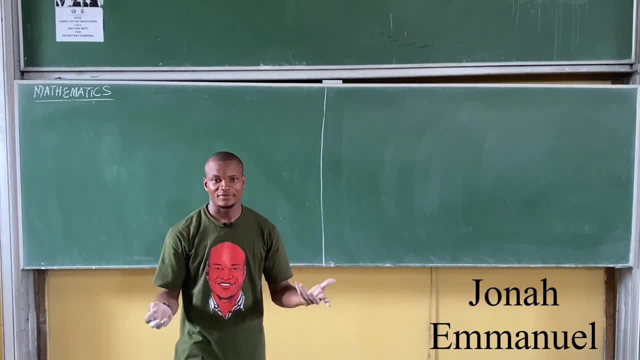 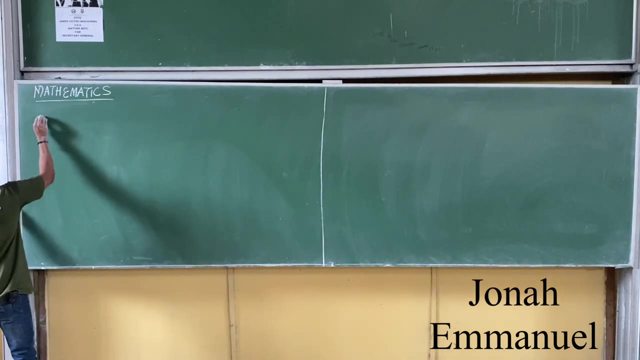 the sign in between the terms are usually positive. so what happens if I have a negative term? what happens if I have a more complex term than just a and b? how do I evaluate it? let's say, for instance, I'm actually evaluating the value of, let's say, 2x. 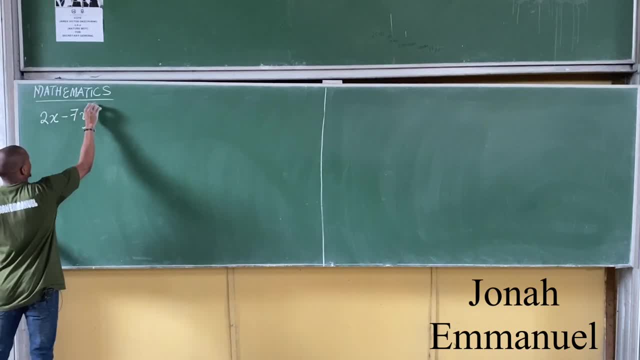 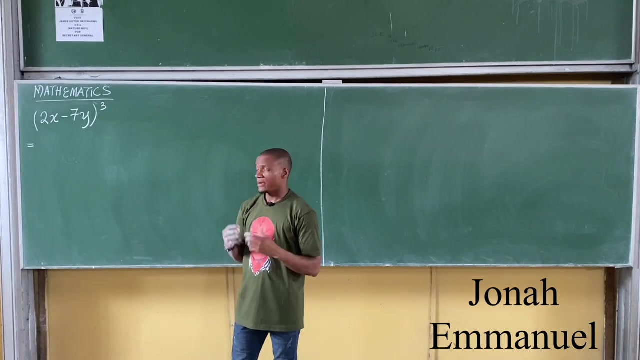 minus 7y, all to the power 3. alright, so what if I'm actually evaluating this using binomial expansion 1y? alright, at this point. choose any convenient method for you. as for me, I'm working with Pascal's triangle. I think that's like best for me. 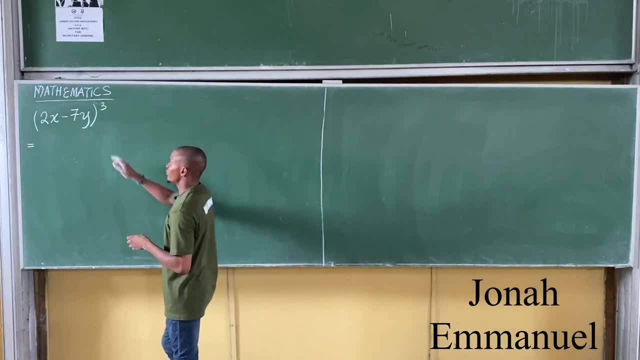 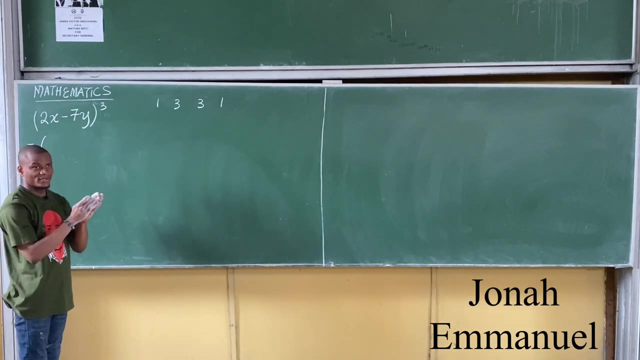 so I work with Pascal's triangle. when it comes to Pascal's triangle for degree 3, my coefficients are what there? 1, 3, 3, 1, so note this alright. so what's the idea there? we sign for expansion such as this. we say the first term. 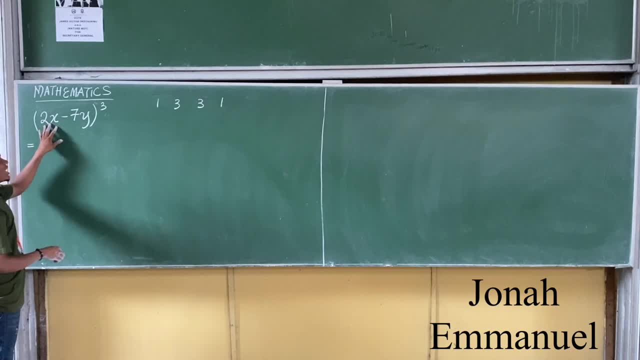 takes all the power. my first term here is now 2x, not just x to become 2x. so 2x here first term takes all the power. that's 3. second term that's minus 7y. minus 7y is less than. 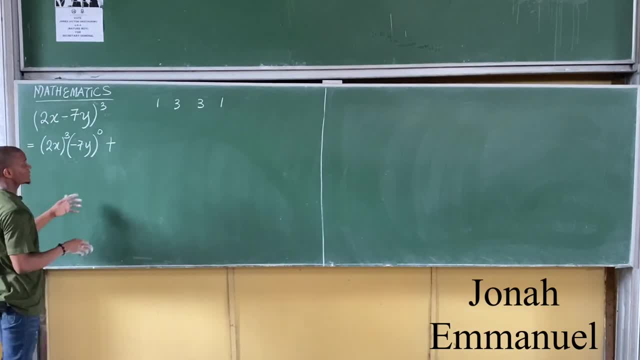 nothing. that becomes 0 plus the same concept. I will increase the power here by 1, so it becomes 2x to power 1 or 2. that's 3 minus 1 is 2. next up minus 7y to power 1. 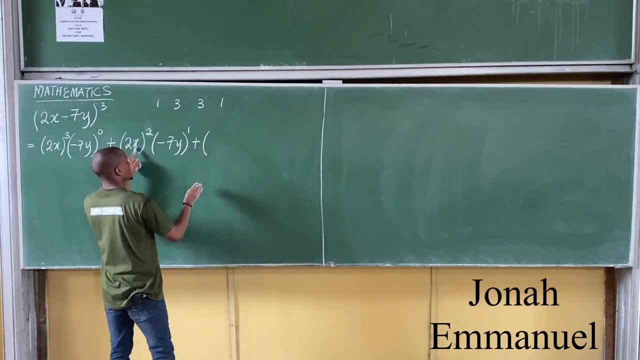 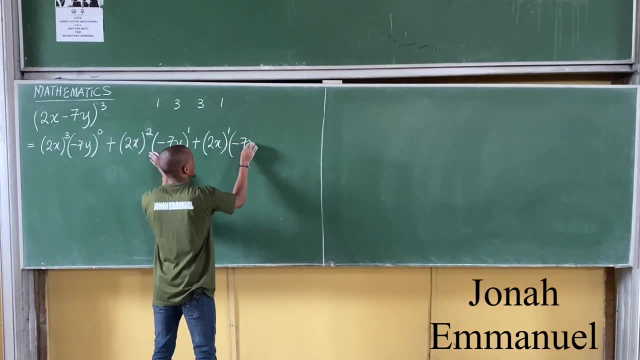 increases by 1 plus reduces by 1 becomes 2x to power 1. increases by 1 becomes minus 7y to power 2. finally, reduces by 1 becomes 2x to power 0 and the last term here becomes minus 7y to power 3. 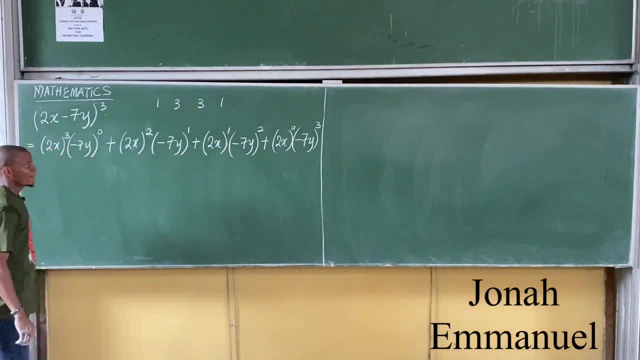 minus 7y to power 3, so it happens alright. so 2 to power 3 gives you 8. next up, x to power 3 gives you 8x. cube d to power 0 gives 1 plus 2 squared gives 4. 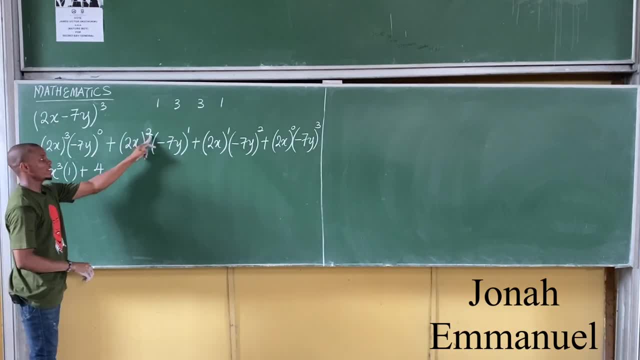 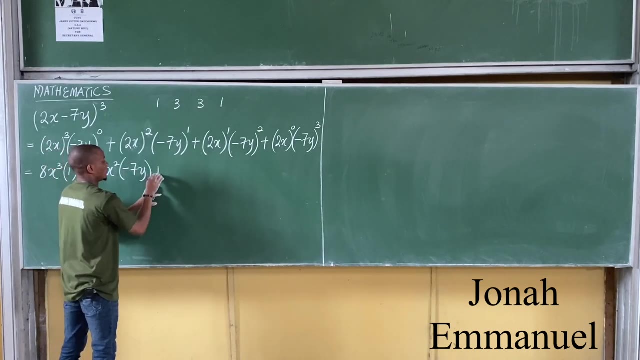 now, mind you, this one affects each of the terms alright. so 2 squared gives 4 this, and this gives x squared d to power 1 is itself alright. any term to power 1 is that same term becomes minus 7y, plus d to power 1 is. 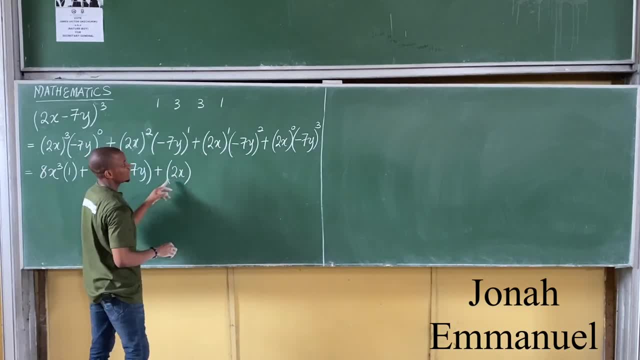 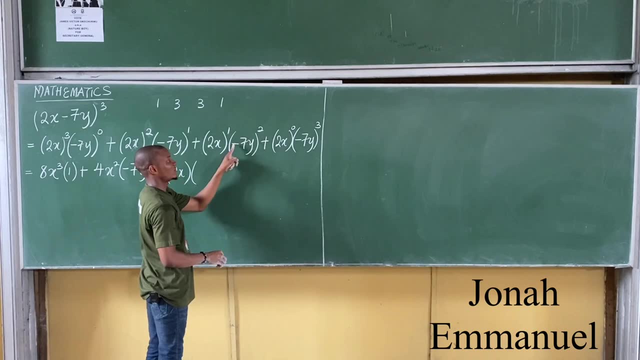 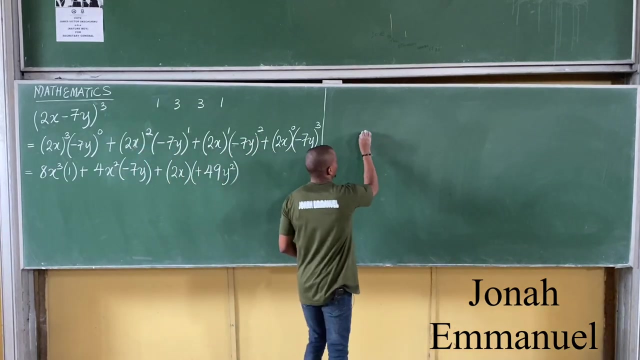 itself, as we said earlier. next up: minus 7 squared, minus 7y, all squared. of course, d squared affects the minus. so minus times minus is plus 7. squared is 49 y squared. alright, if you are unsure of this, if you just come here and see. 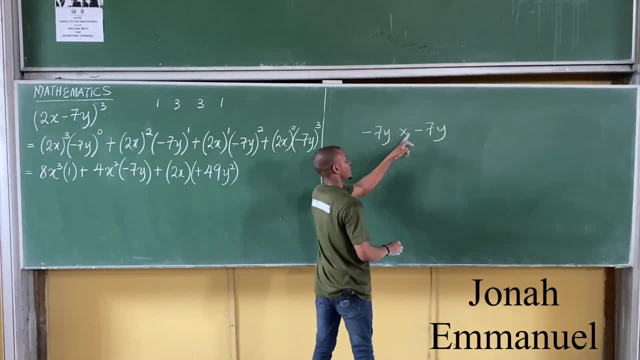 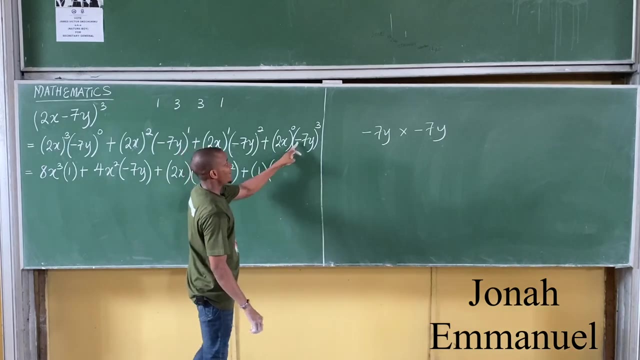 minus 7y times minus 7y minus times minus is plus 7 times 7 is 49 y times y is y squared plus d to power, 0 is 1. finally, minus squared means minus times minus that's plus, times minus that's minus. 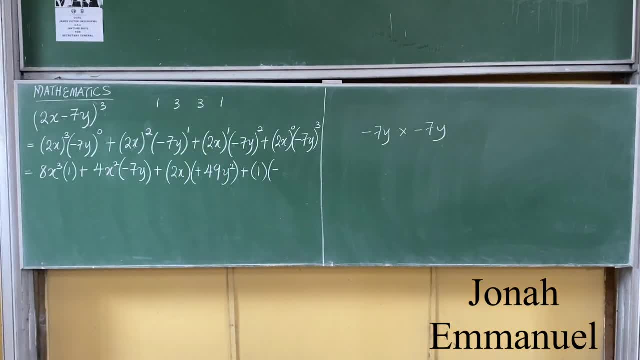 so minus squared is minus 7 squared gives you what? sorry, 3 plus 2, alright. so 7 squared gives you x and this y cubed, alright. so expand this. this is now equal to this: times 1 is itself ok. plus minus is minus. 7. times 4 is 28. 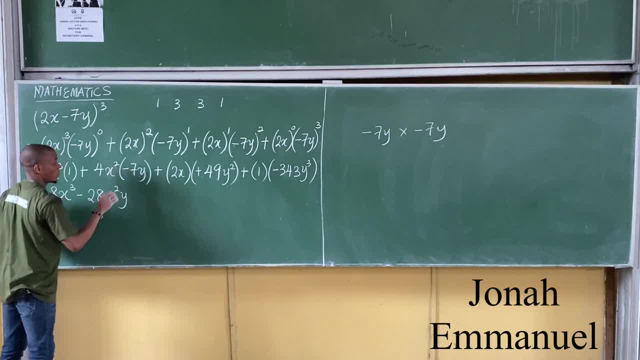 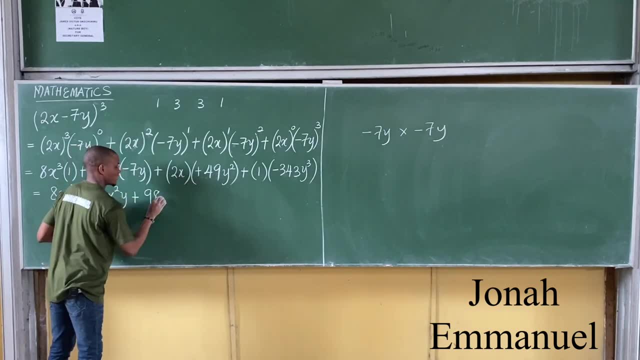 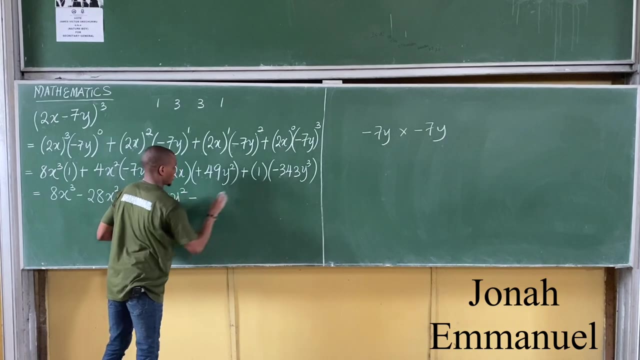 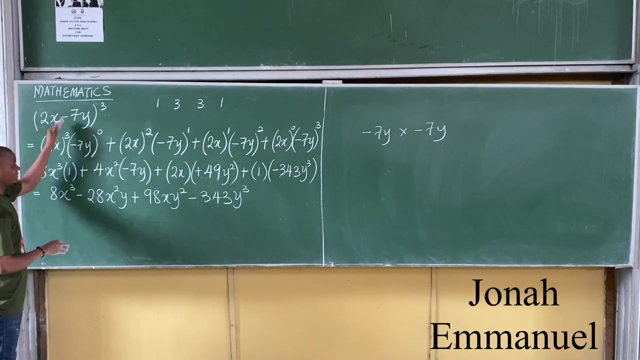 x squared y. x squared y plus 2 times 49 is 98. this and this x- y squared times minus is minus 343 into y cubed. so I have this now. this is my value after expansion. I have not yet included Pascal's coefficient, so after expanding this,